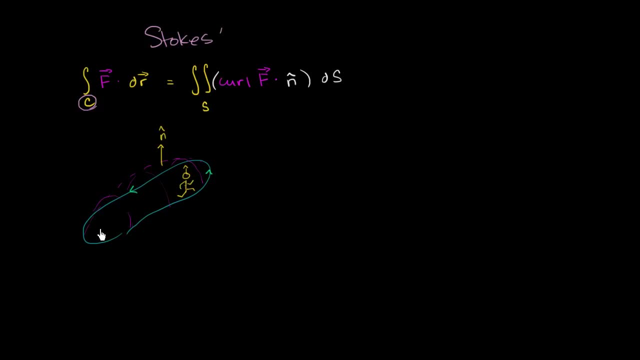 So he would have to go. he would have to go just like that If we oriented the surface differently. so let me redraw the surface right over here, draw a similar surface. So if we had a surface, so this surface looks very similar. 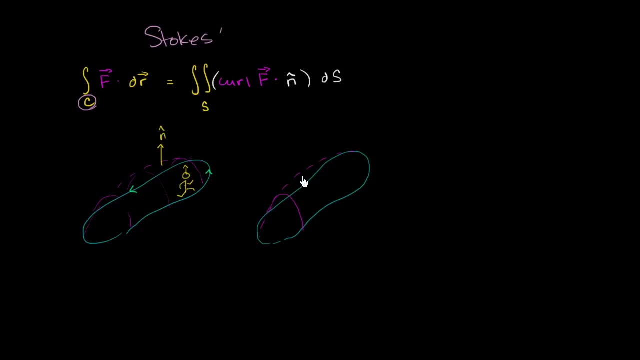 If this surface- so this is a very similar looking surface that I'm drawing right over here just to give an idea of some of the contours- But if we said that the normal vector for this surface we oriented in the opposite way, so if we said that the normal vector here was actually pointing downward, like that, 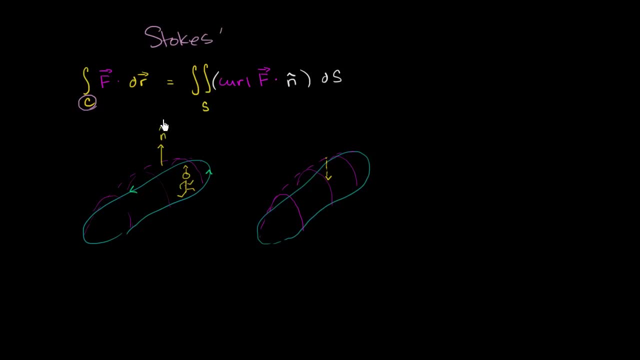 then we would have to- in order for Stokes' theorem to hold, we would have to traverse the boundary in a different direction, Because once again, if I draw my little character right over here, his head is pointed in the direction of the normal vector. 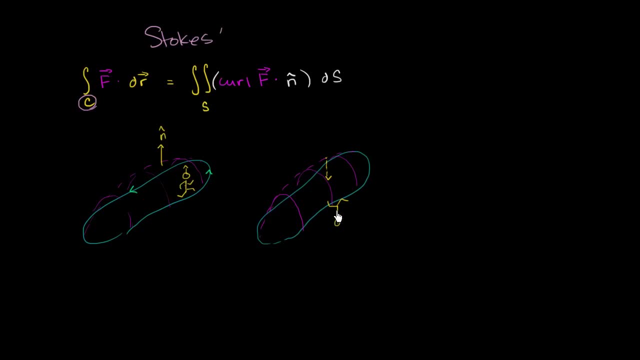 He is now upside down, so let me draw him. So this is him. this is him running right over here. I could draw a better job. This is him running right over here Now, in order to keep, and from his point of view. 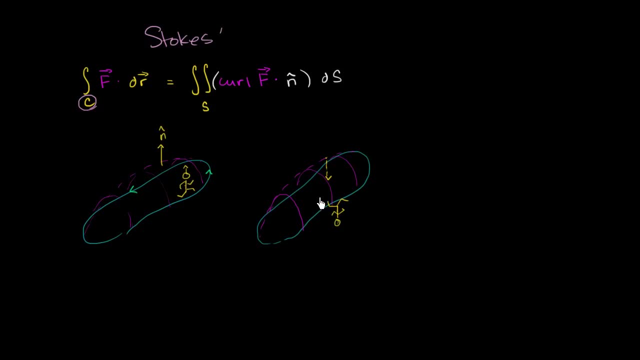 this would kind of look like some type of a pool or a ditch of some kind. It would actually go down Here. it looks like a hill to him, But since he's upside down in order for him to keep the boundary to his left, 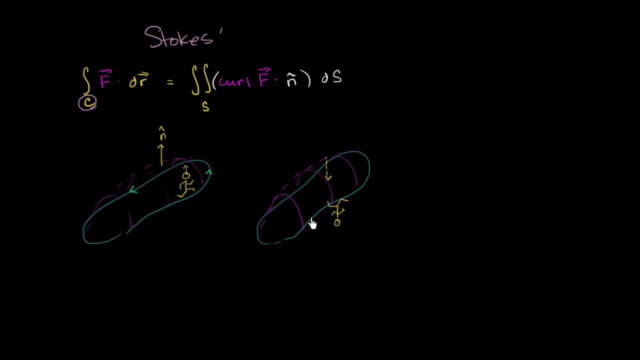 he would have to now go in the other direction. So, depending on the orientation of your normal vector, which is really the orientation of your actual surface, will dictate how you need to traverse the path. Now, another way to think about it, and this idea was introduced by one of the viewers on YouTube. 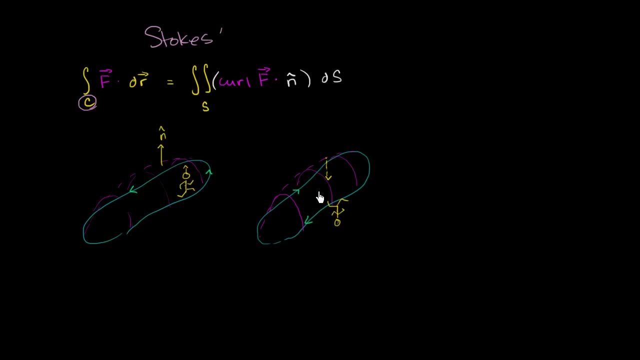 but it's a valid way of thinking about it is to imagine that the surface is a bottle cap And so let me draw some type of a bottle over here, So I'll draw a bottle. So this is, you can imagine some type of a glass soda bottle. 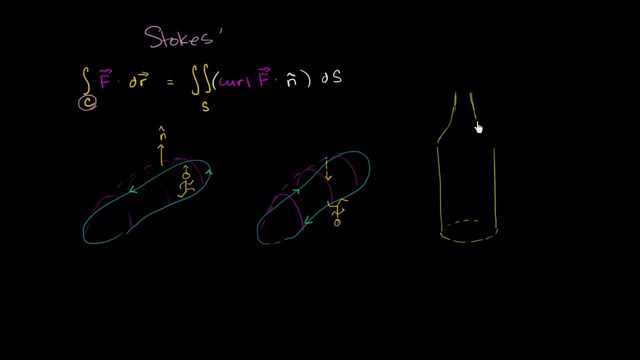 So what we really care about is the cap of the bottle. So let me make it feel like this, Like it's glass. So there, that's our bottle And let me draw its cap. Let me draw the cap of the bottle. 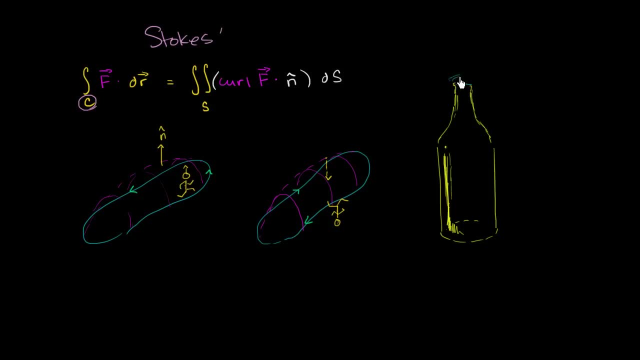 because that's what we care about. We can kind of imagine that being the surface. So this is the cap of our bottle, And you just need to think about. well, which way would I have to twist the cap in order to make the cap move up?